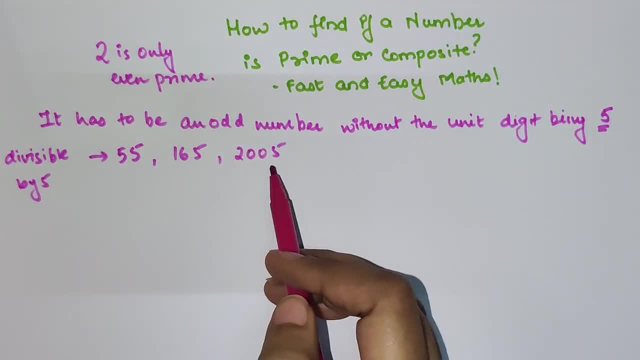 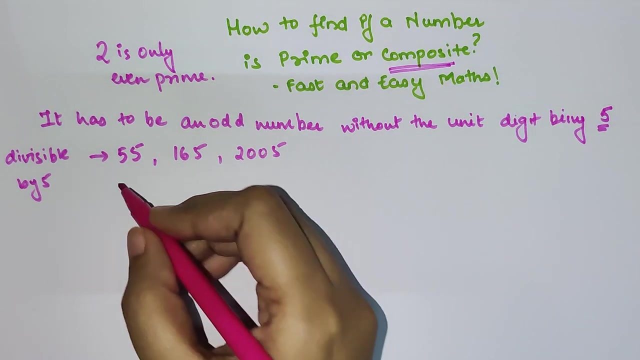 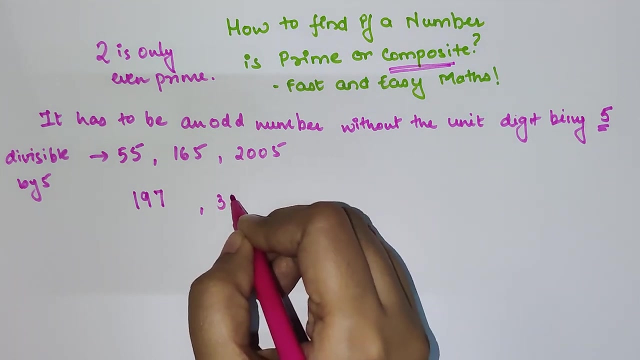 It cannot have any other factor. And if you look, all of these have a factor of 5. So definitely these come into the category of what composite numbers. OK. Now, apart from this, how will you judge that a number which I have given? let's say I give you a number of 197, or let's say 301.. 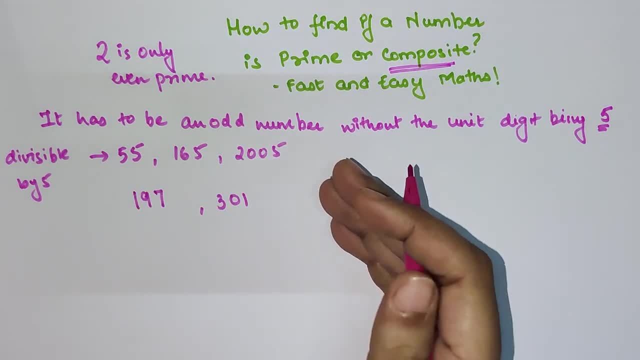 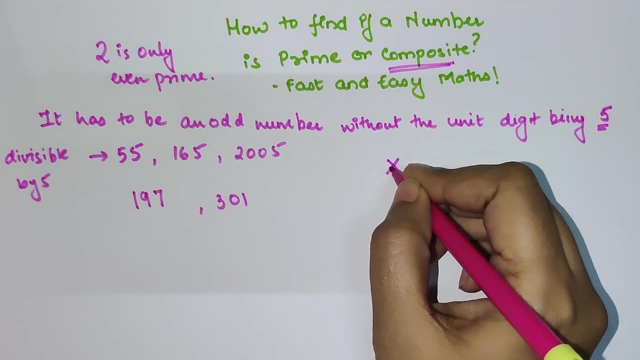 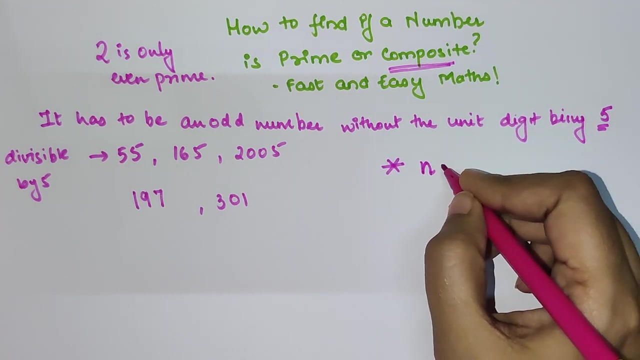 OK, In that case, how will you figure out that, whether this number is divisible, or rather is a prime Number or a composite number? So here, very, very important rule: what you have to do is the number, whatever you have, whatever the number they have given you, if you add 1 to it or if you subtract 1 to it. 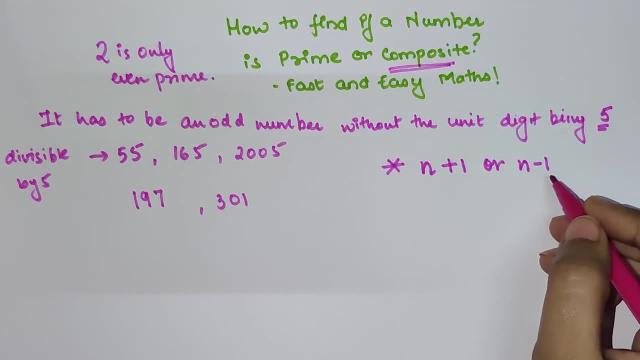 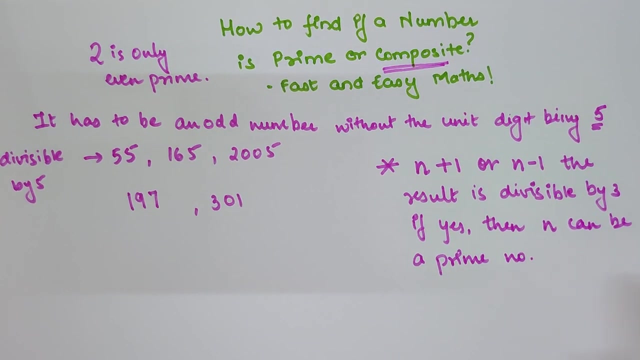 OK. After adding 1 to the number, or after subtracting the number by 1, the result is divisible. OK, OK, So basically, let's add 1 to this. So when you add 197 plus 1, what you get is 198.. 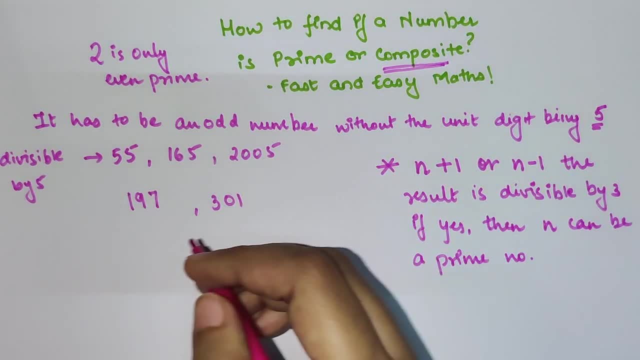 OK, And 198 is basically coming out to be when you let's check this. So if you get 1 to 1, you get. if you get 1 to 1, you get. so if you add 1 to 1, you get 99.. 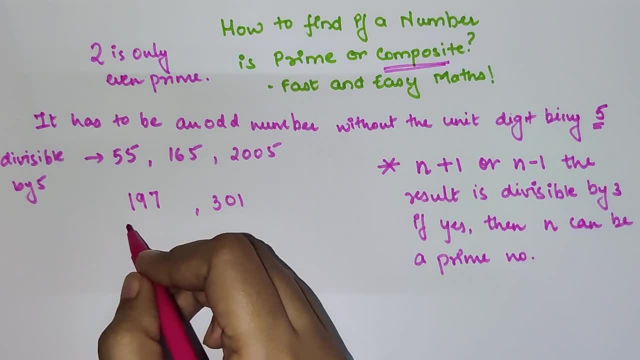 Then you get 99.. the divisibility rule for 3 is what? adding all the digits? so here let's just add: either we get 198 or we get 196. okay, so now what is the divisibility rule of 3 that you have to add? 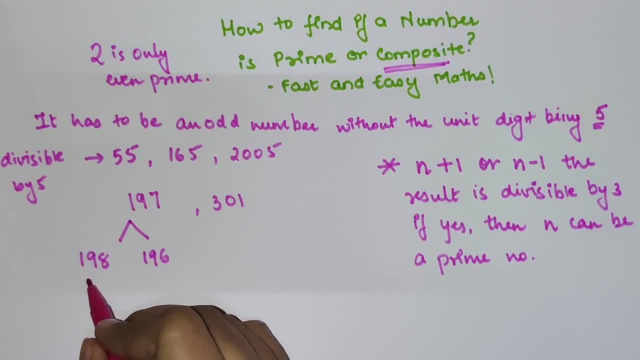 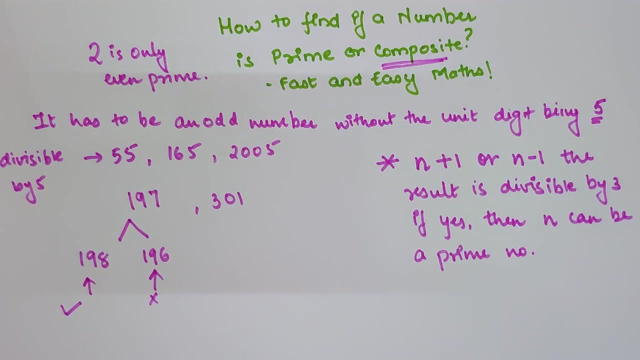 all the digits. and when you add all of this, all of these digits, it is what divisible by 3, and this is not okay. but whatever i said, that either one plus 1 or minus 1, any of this is divisible by 3, then we can say that the number can be a prime number, but please understand the emphasis on cap. 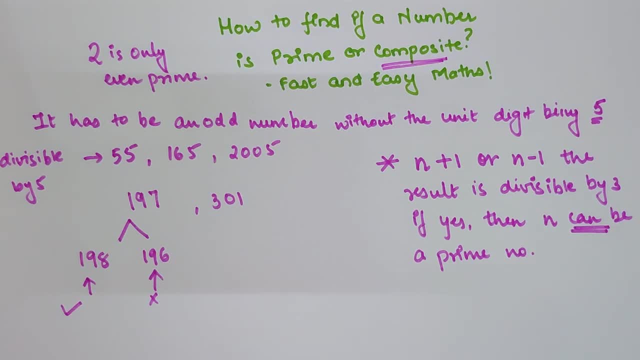 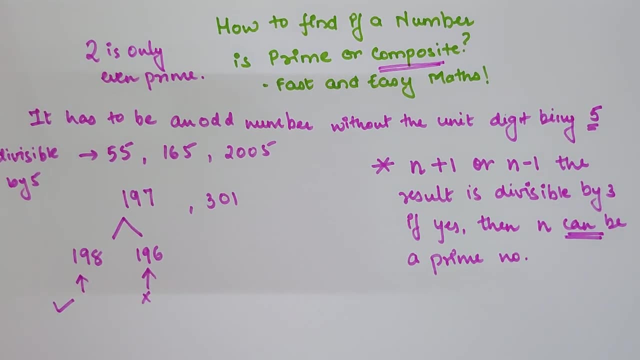 can be. it is not necessary that it will for sure be a prime number. i will very soon show you an example where it is being divisible by 3, but still it is not a prime number. in this case, what you do is you, if you want to be like completely sure, what you do is: first you take 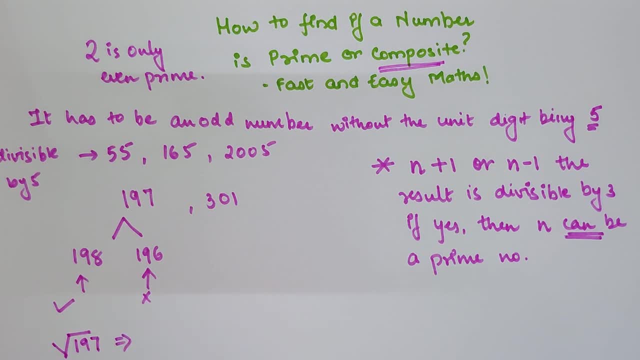 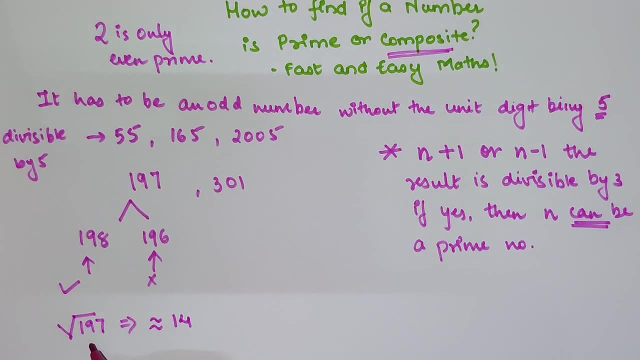 square root of 197. square root of 197, can i say it is very close to 14, so i will check whether this number is divisible by all the night prime numbers, which is leading up to 14. so how many prime numbers are there? two, three, five, seven, eleven and thirteen? okay, why i haven't taken 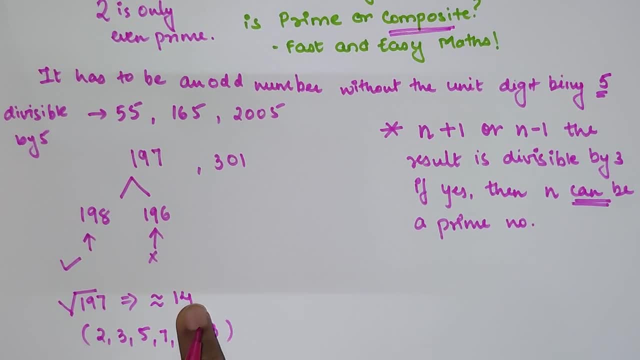 the square root of 197, because it is very close to 14. so i will check whether this number is divisible. anything other than that, because we are just going to take number prime numbers up till 14 means the number whatever they have given you. you have to take the square root of it. 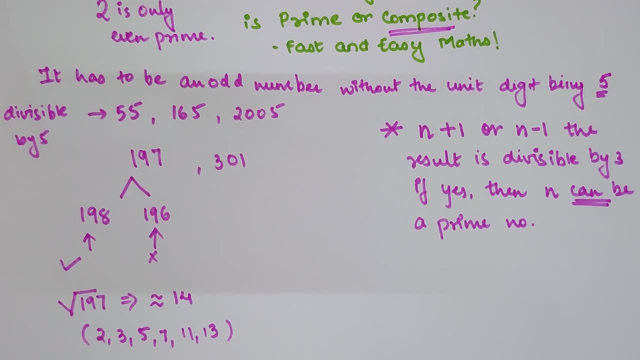 and then you will try, or rather you will test for the divisibility rules of all the prime numbers resulting up to that particular number. okay, so now, since this is obviously an odd number, so this is not divisible by two. three also, it is not divisible. five also, it is not divisible for seven. 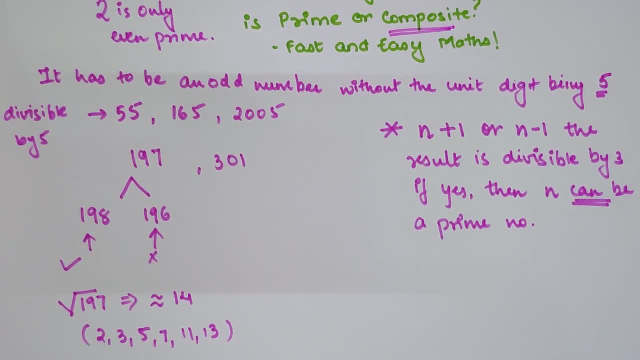 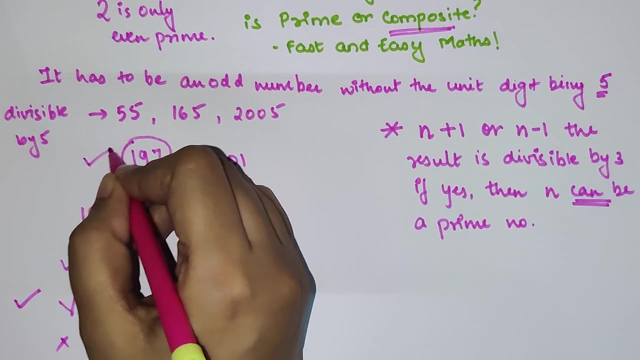 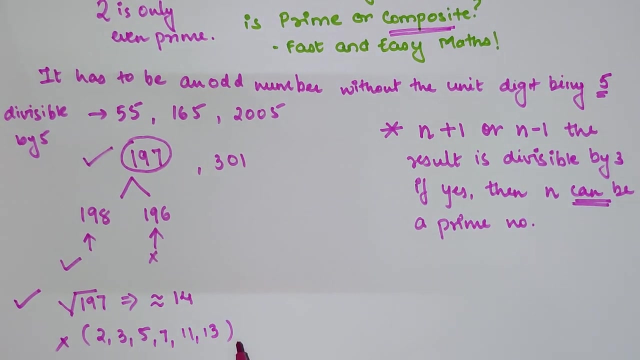 um, no, for seven also, it's not divisible. 11, no, and 13 also no. so i can say that, yes, this particular number is a prime number, or rather, this number 197 is a prime number. understood. now i understand. for in order to know what are the divisibility rules of 7, 11 and 13, i have made a separate video. 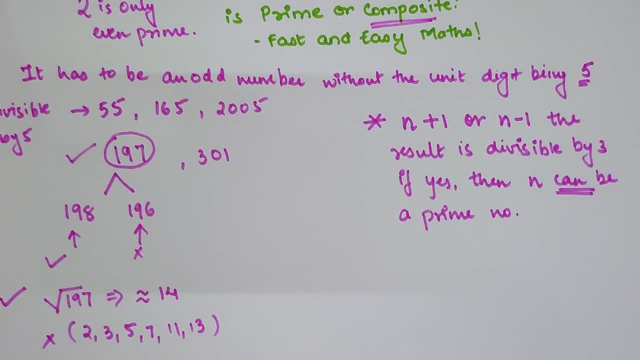 on that. so please go ahead and check it out and i will see you in the next video. bye, bye, bye. check that out. i'll put the link in the description or in somewhere on the top. you will get that link. okay, now coming to this. so again, when you do this, so we get 300 and 2 or 300. so 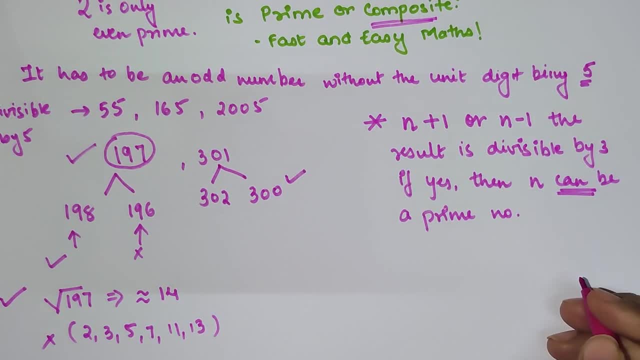 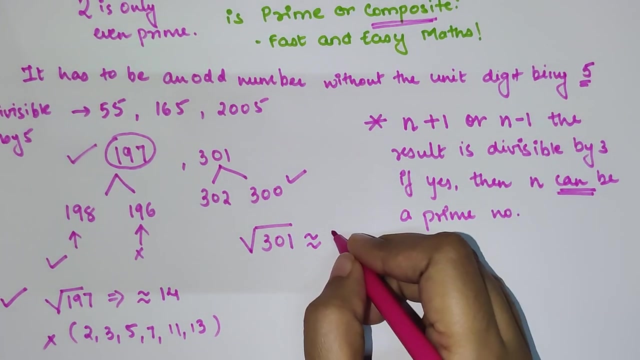 now this is divisible by 3. okay, so now let's check for the divisibility rule. so now let's take square root of 301. so this is very close to, let's say, 17. so again we will check for all the prime numbers leading up to 17. so that is 2, 3, 5, 7, 11. 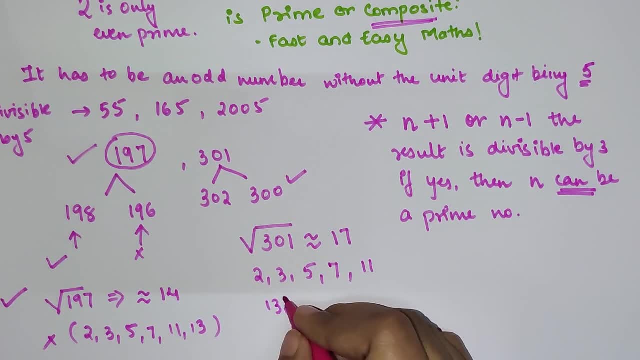 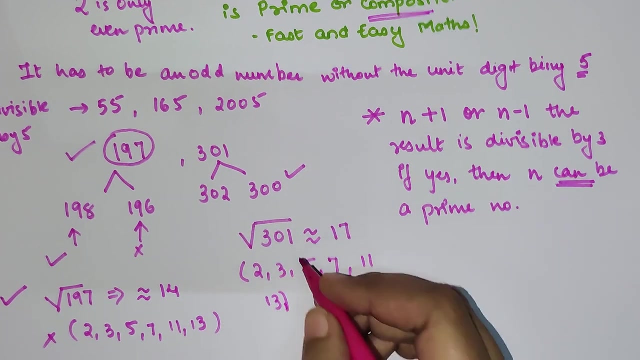 13. yeah, that's it. so again, we will check for all of these prime numbers. so again, 2, 1, 3 is gone. 5 is also gone for 7. um, if you don't know, i'll tell you what is the divisibility rule for 7, that is: 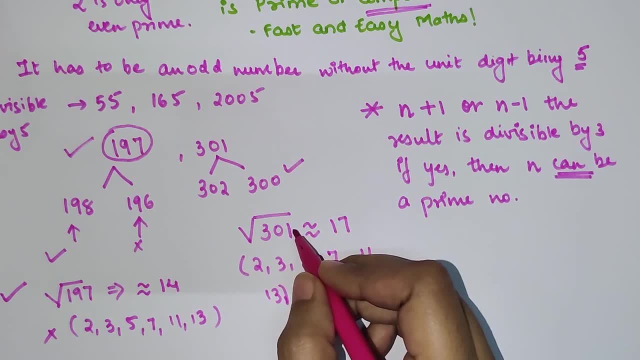 multiply or divide by 7. so this is the divisibility rule for 7 and this is the divisibility rule for 8, or rather double the last unit digit. so which is what? 2? 1 into 2 is 2 and you subtract whatever. 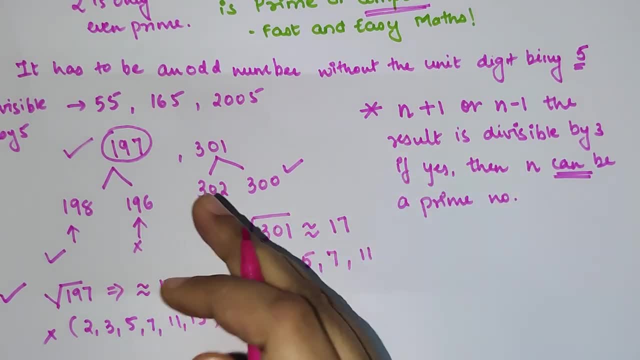 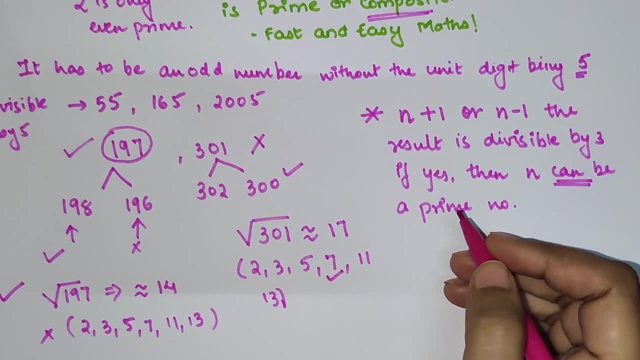 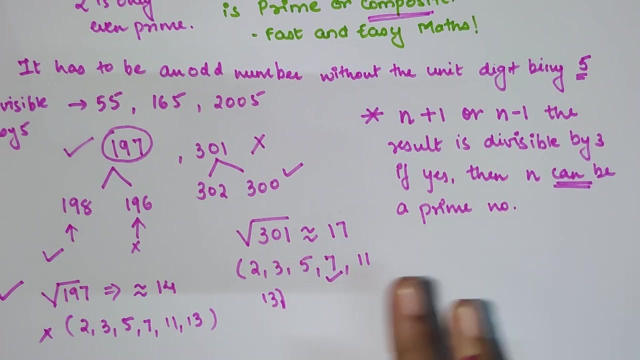 answer you get from the rest of the digit, which is 30. so 30 minus 2 gets you 28 and, yes, it is divisible by 7. so we can say that this is not a prime number. so you understood, in both these scenarios they were being divisible by 3, but one of it was not was a prime number and other was not. 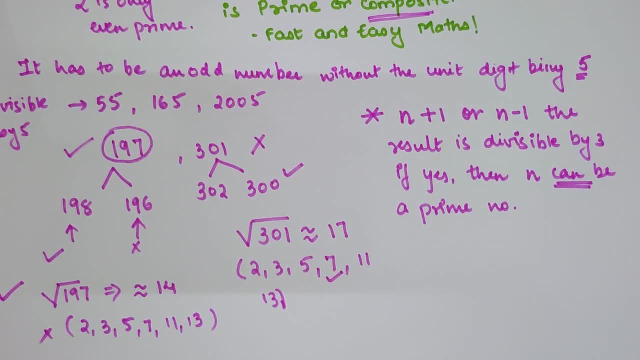 so, in order to be, in order to be completely divisible by 3, but one of it was not- was a prime number and other was not. so, in order to be sure, in that case, you have to use this particular logic of taking the square root. okay, so now very. 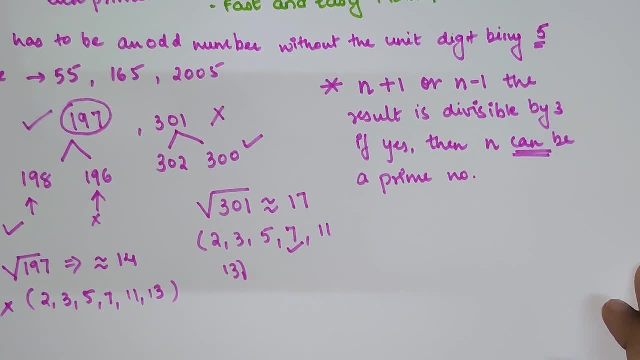 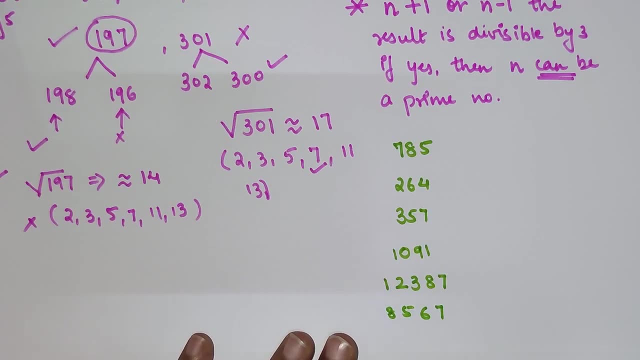 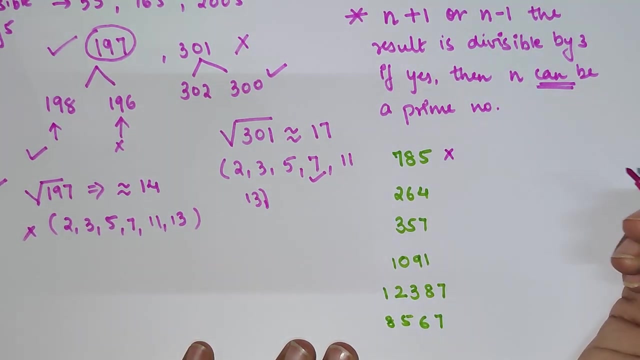 quickly, let me write down few questions and let's see whether you will be able to figure out whether they are. they are, they can be a prime number or a composite number. so here i have given you a list of numbers. so now, from here, looking at these two, this number, we can directly say it's not a prime. 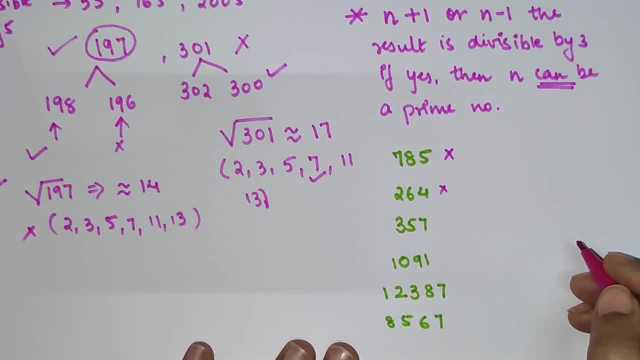 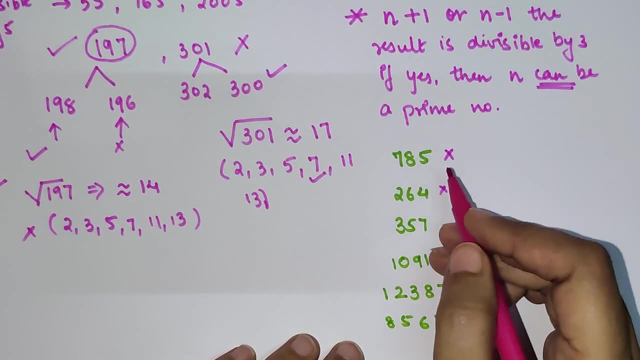 number. it's a composite number. this is also not a prime number. it's a composite number. okay, why? because this was an even number and this number, even though it is it- was odd. it still had the last digit, which was 5. that means it has a factor of 5. okay, now the next one. so here we are. 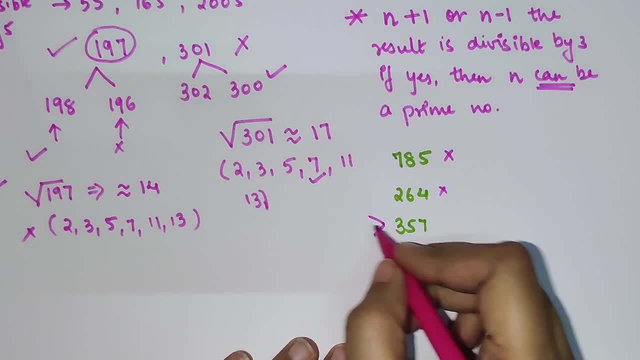 going to do plus and minus 1, so 357 minus 1 will get you 356 and plus 1 will get you 358. so now, 3 plus 5 is 11. sorry, 3 plus 5 is 8, 8 plus 6 is 14 and 3 plus 5. 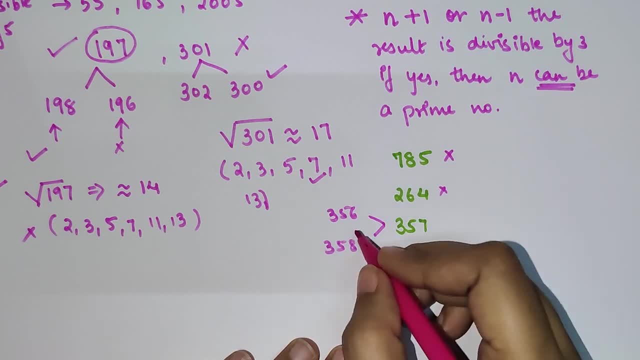 is again 8. 8 plus 8 is 16. so here we can say both: the plus 1 minus 1 is not being divisible by 3, so we can directly say that this number is not a prime number. over here we get 1090, 1092, now over.